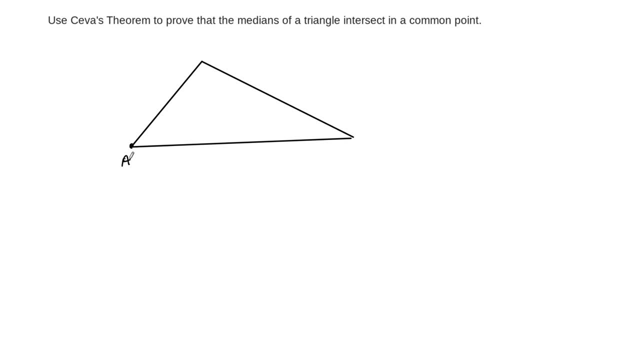 though, so you can make this triangle however you want, And I'm going to label these vertices- A, B, C, in this direction. And at this point, the median- remember the medians- of a triangle are the segments, the line segments that connect the midpoints of each side. So let's. 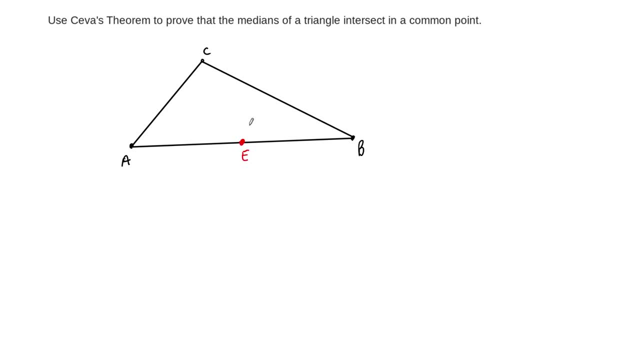 call this one. let's call this one E. So this is. the idea here is that this is the midpoint, so it divides us evenly, right. So E. and then let's call this one F. By the way, I'm just 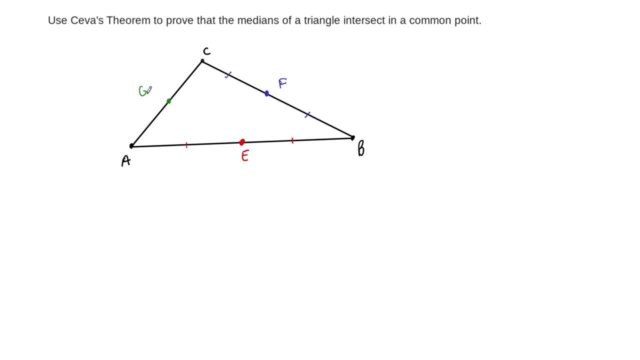 eyeballing this. I'm not constructing this, but I'm just eyeballing it. So E, F and G. So there's the idea. And then E, F and G. Now we can connect these points to their opposite midpoints. These are the medians. 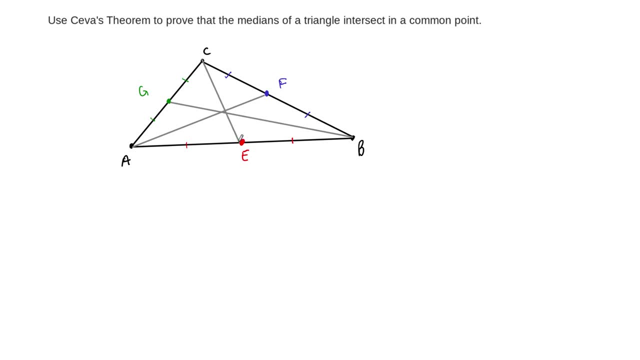 now And hopefully this goes through. If not, we're going to use what's called a big point theorem, because I didn't measure anything. So the idea here is that these should all go through this common point, this common point D, if I had chosen the points correctly. 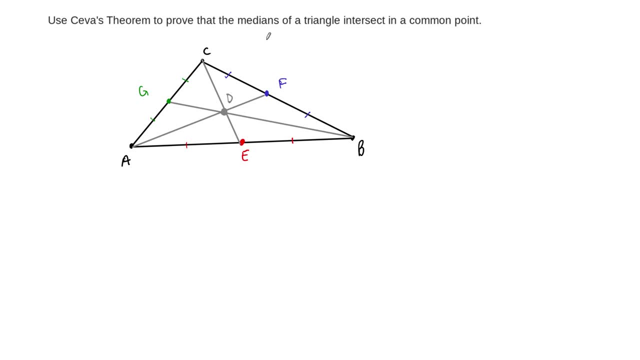 right. So it's a little bit off, but that's okay. So here's the picture that we want to prove. We want to prove that these all intersect in this common point D. So that's to be proved right. I'm not going to write this proof as a table, I'm just going to work through the. 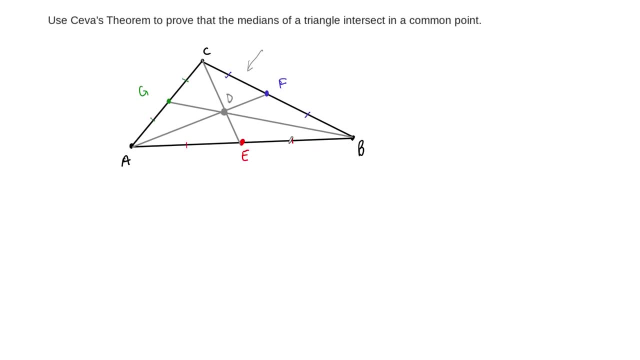 argument. So we see here that we have these equal side lengths, right. So AE, remember side lengths. we don't draw the bar over it, right? But the measure of side of this segment, AE, is equal to EB. And by the way- I'm going to go around counterclockwise- We haven't. 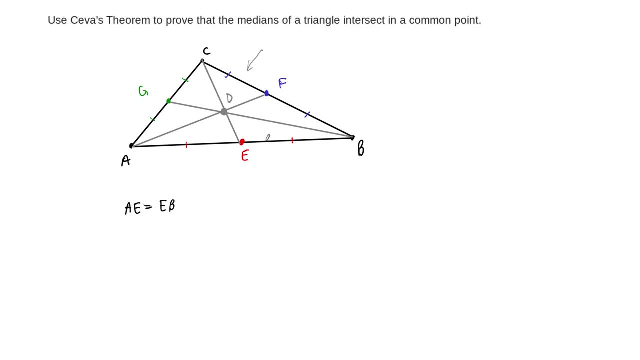 talked about this, but in terms of positive I'm going to go around counterclockwise. So positive versus negative. if you reverse the order, so EB is equal to negative BE. So once you switch the order you get a negative sign. That's the convention in geometry. So 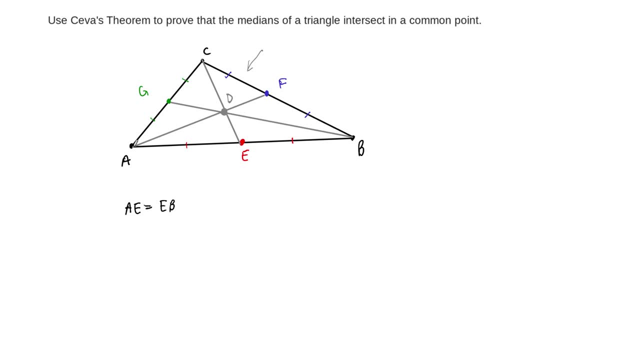 I'm going to go in the same direction around this entire triangle. And then what do we have? Well, the next one we have: BF is equal to FC, right? So these two are equal because of the median property, the midpoint property. And then we have CG is equal to GF, is equal to GF. 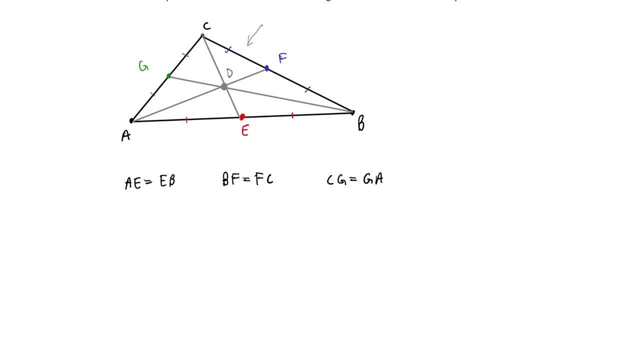 All right, So once we now get to Siva's theorem. so Siva's theorem says that we should take the ratios of these portions of the side length and then multiply them all together. right, So we have AE divided by EB times, BF divided by FC times, CG divided by GA. All right, And 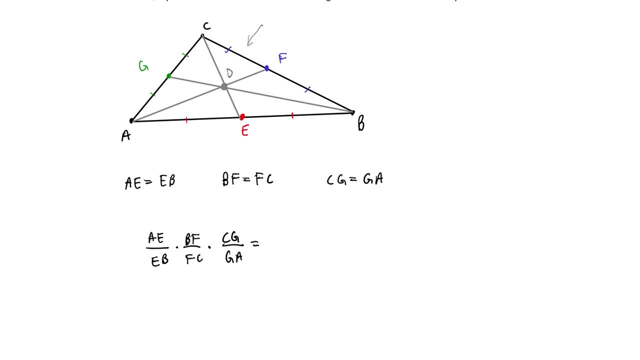 this. we need to now compute right. But look at what we have here. We have BF divided by EB times- BF- All right. So we have BF divided by EB times- BF- All right. So we have AE and EB. They're equal. So this cancels out, leaves us with one Same thing on the next one: BF. 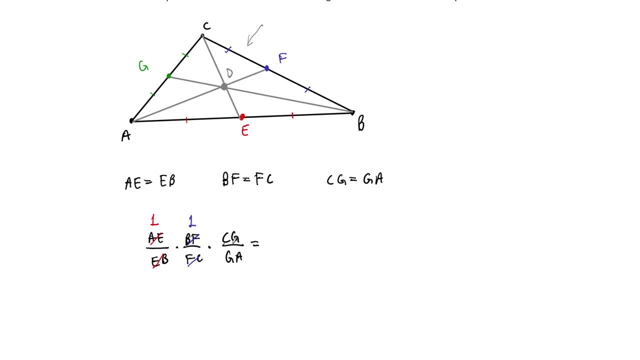 equal to FC. That's a one right. Same thing on the last one: CG equal to GA. So that ratio is equal to one And this product just becomes one times one times one. Therefore, the product of the ratios of these sub side lengths right is equal to one. And then Siva's theorem tells: 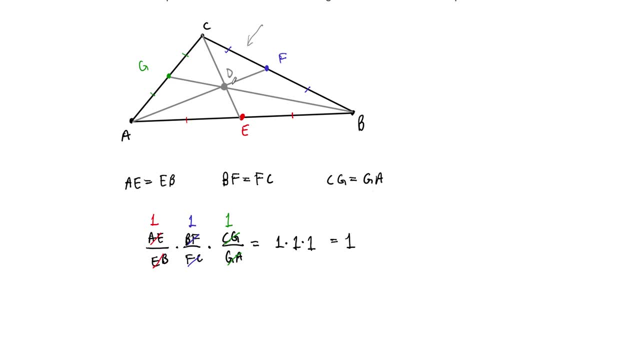 us, if BF is equal to FC, then it's equal to GA, So that ratio is equal to one And this product is one. If the product of these ratios is one, then the line segments that connect the opposite vertex to that point, those lines must be, they must intersect in. 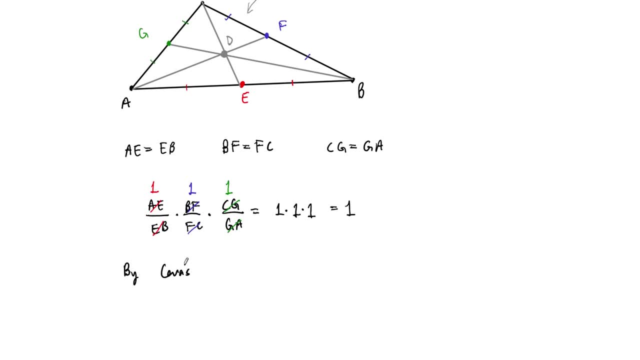 a single point right. So now, by Siva's theorem, these line segments which happen to be the medians. right because of the way that they were constructed. So, by Siva's theorem, the lines AF, BG. 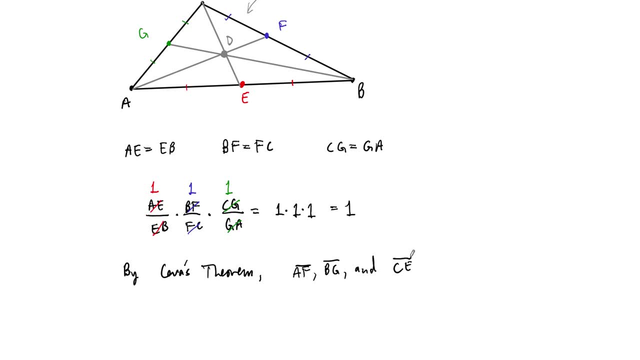 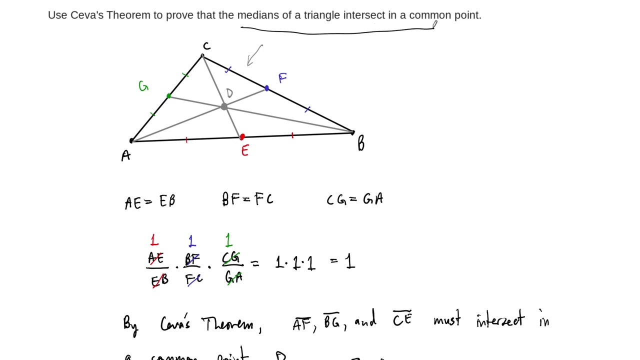 And CE must intersect in a common point, And that common point in my picture is D, right, So there we go, And so there's the argument. We're going to call that a proof And that proves that the medians of a triangle, the medians of a triangle, intersect in a common 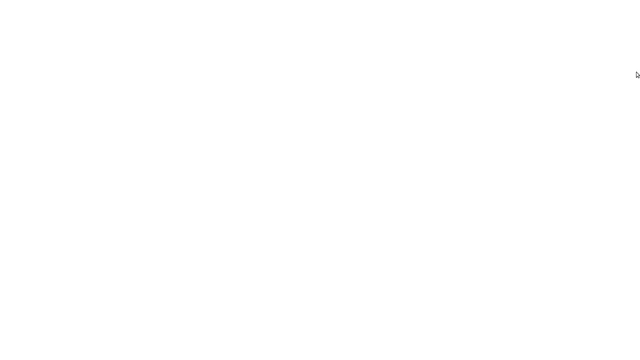 point. Now, I'm sure you guys are familiar with this. I'm sure you guys are familiar with this. I'm sure you guys have thought through this. But that requires, then, that we believe Siva's theorem, right? So it turns out that Siva's theorem is true, But Siva's theorem is doing 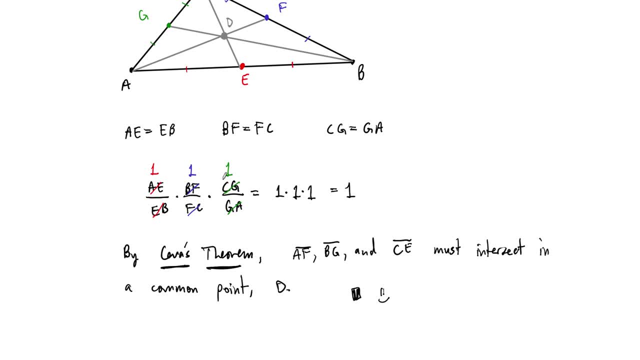 all the work here. We just did a nice little calculation to get that the product of the ratios is one. Siva's theorem did the rest of the work okay. So there's an application of Siva's theorem.